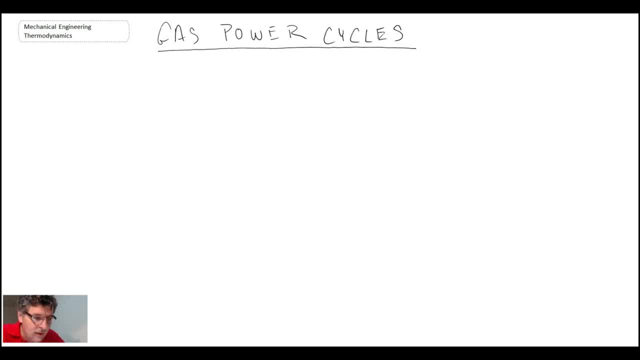 theory that we have thus far developed and all of the tools that we have: property data, the equations. So we're now going to start with gas power cycles, which are probably one of the most common known thermodynamic systems that each of us deals with daily, because 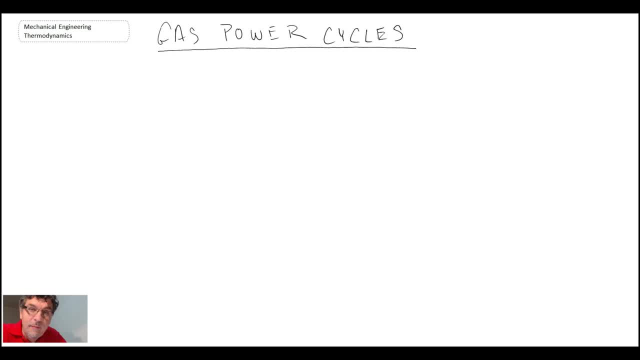 these are the systems that are used to provide power for cars or automobiles, planes, buses, trains- unless it's an electric train, However, if it's using any kind of fuel, it would be using a gas power cycle. So what we'll be doing is we'll be taking a look at gas power cycles in today's 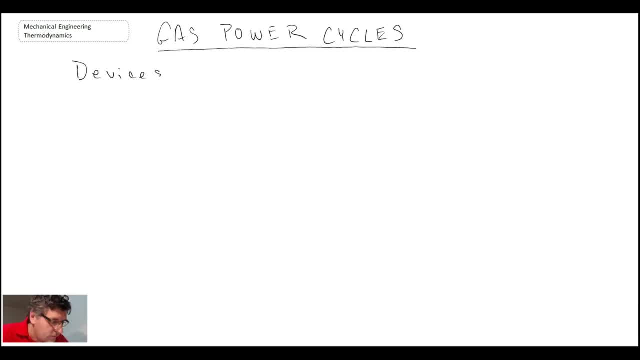 lecture, And so the key thing here is that the gas power cycles are producing power from a heat source, So that's one thing. The other thing to note is that the working fluid in these systems remains a gas. We will be looking at other power cycles later, in the class called the vapor power cycle. 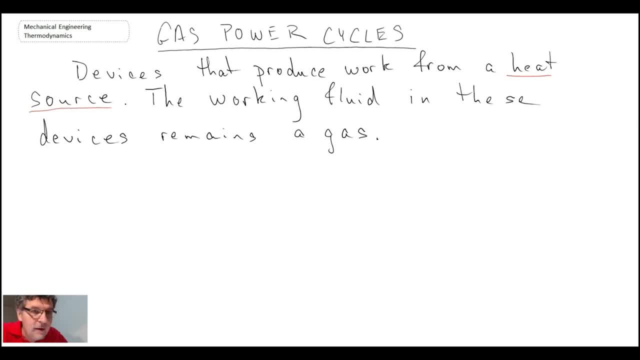 The most famous of that is the Rankine. Rankine cycle is used in steam power plants and steam engines of old, And there what is happening is your working fluid goes through a phase change, So you would go from a liquid to a vapor state. However, here what we're dealing with is a system whereby the working fluid in our cycle 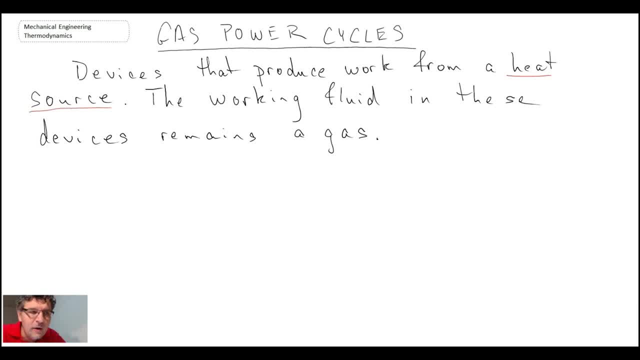 remains in the gas phase. Now I guess technically you could argue that if you have a liquid gas like gasoline or diesel fuel, you're injecting that. But what we do is we atomize that when we inject it into the airstream, And so we can consider the working fluid to be a gas for these cycles. So examples: 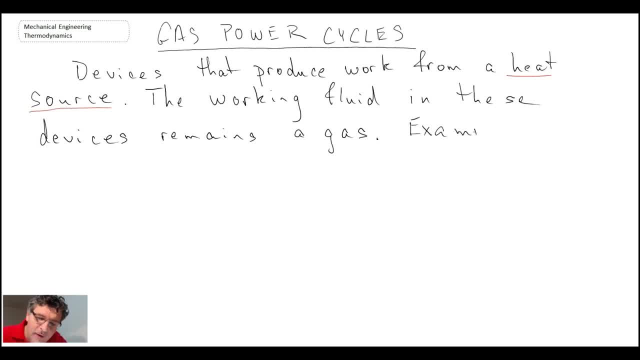 of these gas power cycles would include the following: We have spark ignition engines, And these are engines where you have what we call a spark plug. And what the spark plug is. it's a gap between two metals And you put a high voltage across it and you'll get a spark forming, But that is what initiates the combustion within our system. 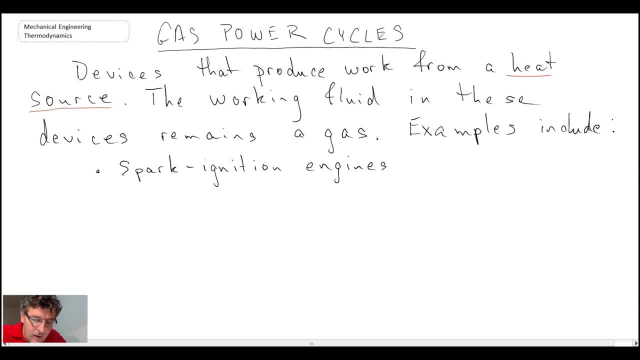 And so, consequently, we call those spark ignition engines, which tend to be quite popular. They're used in a lot of cars. We have diesel engines which, by comparison to spark ignition, these are actually compression ignition engines, And here our pressure ratio is going to be higher, And what happens is you compress the engine and you start to see that the제. 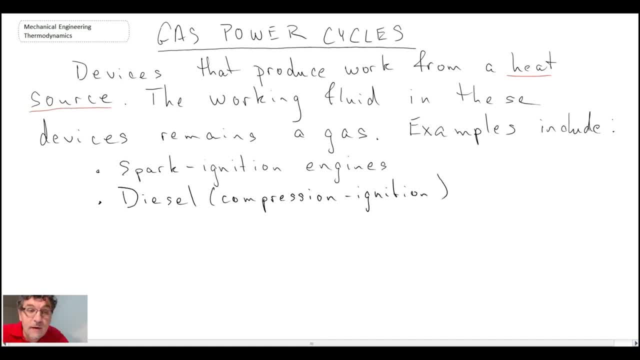 so you can see the ignition é higher and what happens is you compress the, the charge, so the gas fuel, the, the fuel air mixture, to a high enough pressure and there's also a glow plug in these engines. but that will initiate the combustion process. so it's compression ignition engines and in a later 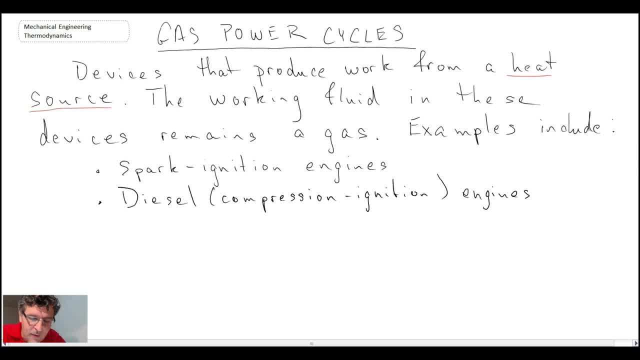 lecture. i'll let you hear these and so you can hear the difference between a spark ignition engine and a diesel or compression ignition engine. Another form which is really a very, very different design from both spark ignition and compression ignition are gas turbines. but these also fall under the definition of gas power cycles. gas turbines are used. 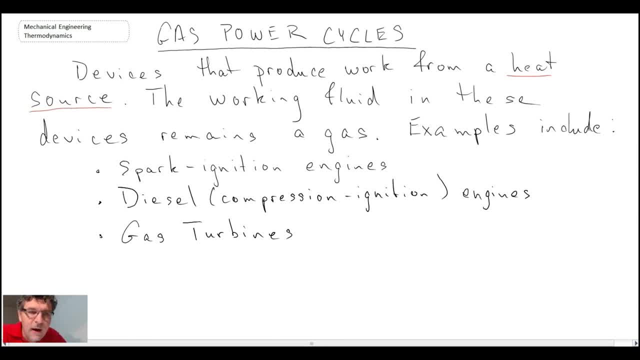 in industrial applications for power generation. but the one that you're probably most familiar with would be the one that's hanging underneath, let's say, the wing of a triple seven or of an 800 unit engine A380.. Those are gas turbine engines and they are what provide the propulsion for the aircraft when 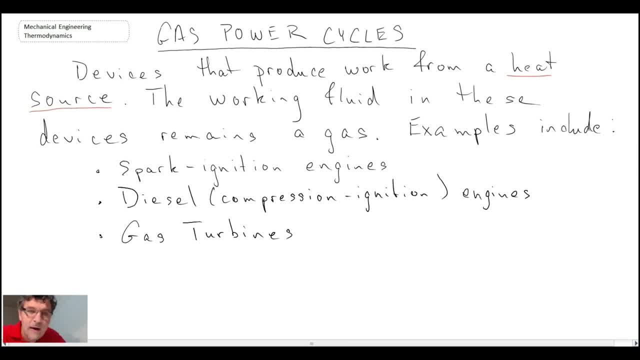 it's flying, but they're also used for other applications. like I mentioned, Gas transmission pipelines use them for power production, Typically when you're above about the 30 megawatt range- that's when you get into the gas turbine engines- but they're also used for stationary power. 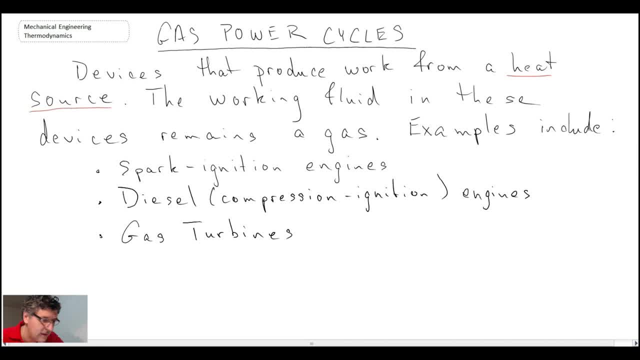 production, peaking power for electrical utilities, things like that. But these engines, all three of these, or cycles, I should say. the thing that is in common here is the combustion process is taking place inside of the engine, And so these are internal combustion. 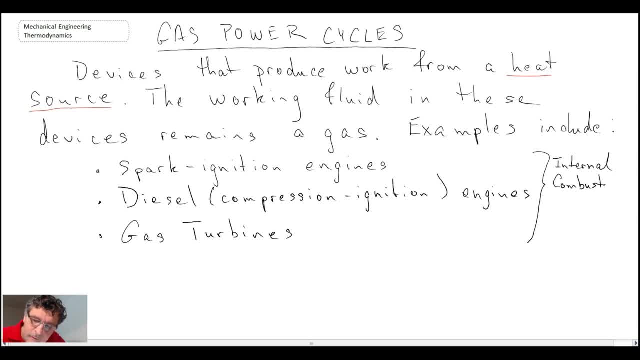 engines or cycles. And that is contrasted by two other cycles that we will study, one being the Stirling cycle, or Stirling engine, and the other is the Ericsson cycle, or Ericsson engine, And these are external combustion engines. And so here what happens is you're burning or combusting, you're oxidizing. 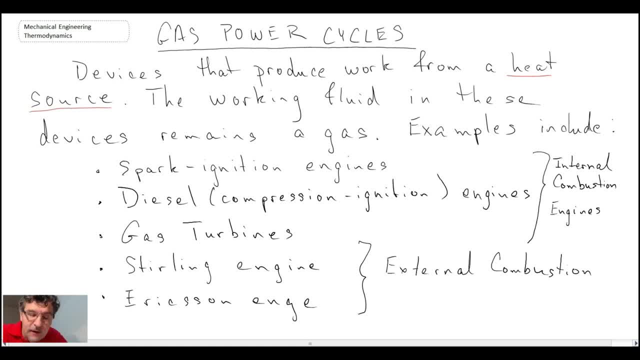 your fuel mixture outside of the engine and that generates the heat which then goes through heat transfer and heats up the working engine. And that's what we're going to talk about in the next video. But that's a different design of engine versus the spark ignition compression. 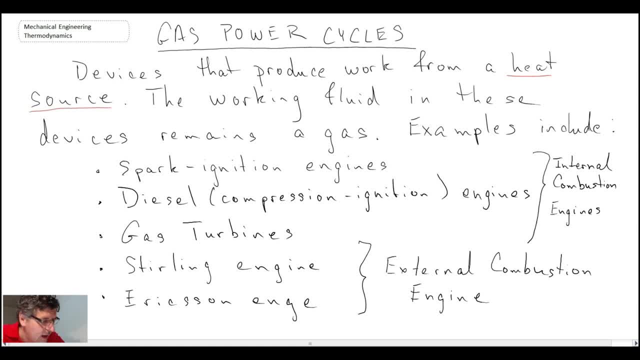 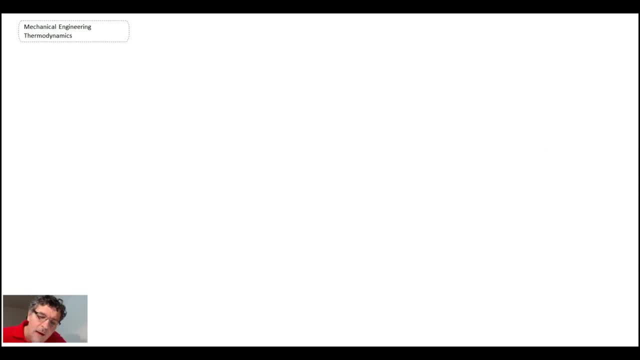 ignition or the gas turbine, which is actually the Brayton cycle. With those you have combustion inside of the engine. So when we're doing our calculations we're going to have to make some assumptions here, because these cycles are very complex And in order to do our basic analysis we need 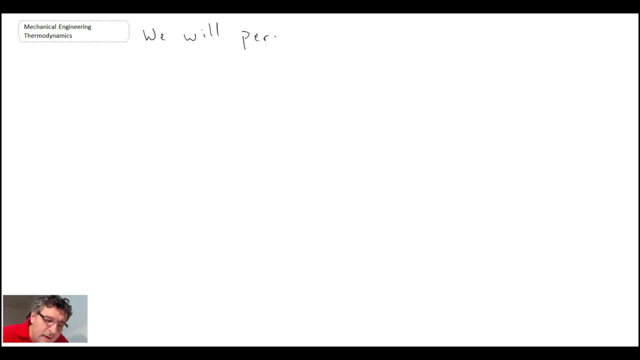 to simplify things. So what we are going to be doing is doing what we call ideal cycle analysis, And I will write down what the different components of ideal cycle analysis are. First, we assume that there is no friction, And by friction I mean both mechanical, So mechanical friction within the moving parts of 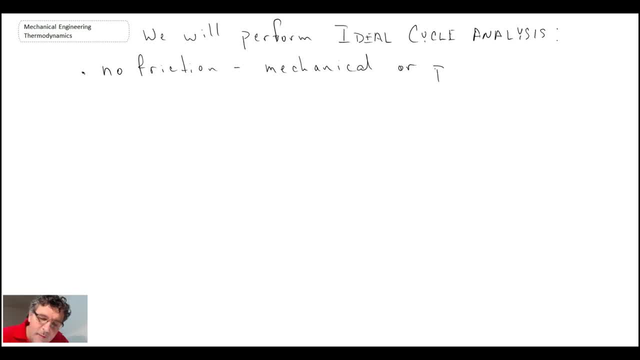 the engine Or fluid friction, so that would be pressure drop as the working fluid moves throughout our engine. So we're assuming there's no friction, We're assuming that things are operating in a quasi-equilibrium manner, And that's typically for our expansion and compression processes. 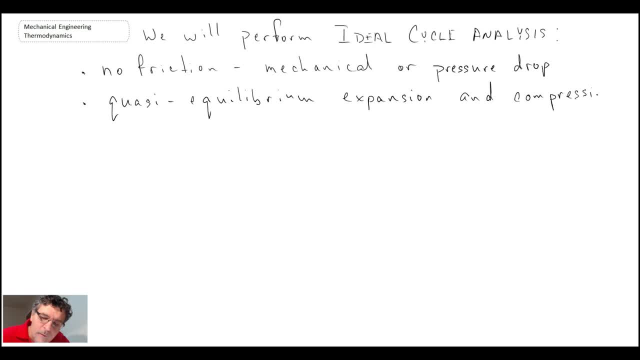 Expansion is where you get the power. Compression: you have to put the work in in order to compress the air or the air-fuel mixture. Another thing that we will assume as part of ideal cycle analysis is that heat transfer is negligible when not intended. 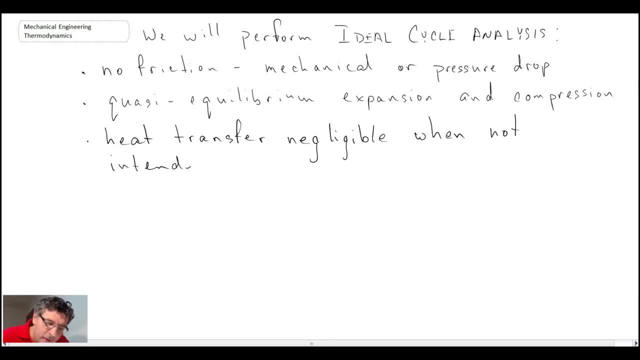 Now we will assume that there is no heat transfer. We will have heat transfer, and I'll talk about that in a moment. That's how we actually heat the working fluid. But where would it be negligible, when not intended? That might be the pipes that are connecting one component of the engine cycle with another. 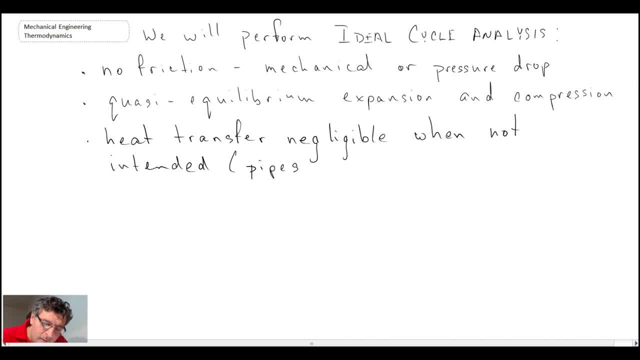 So I'll just write here: pipes connecting components, And another assumption that we will make as part of ideal cycle analysis is that heat transfer is going to be through a finite temperature differential, And what this means is that the cycles that we're analyzing are not externally reversible. 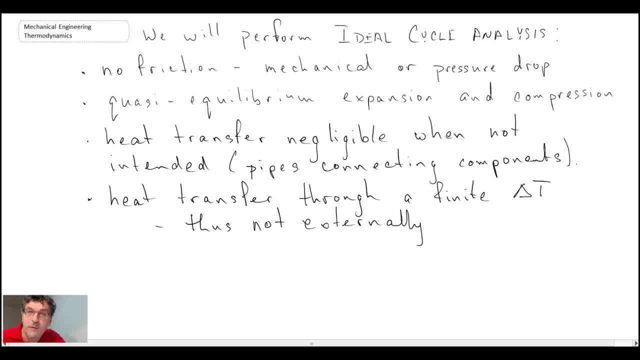 In order to have it externally reversible, we would have to have heat transfer through an infinitesimal delta T, which we said is really not practical for real engines or any kind of cycle that we study. Okay, so those are the things of the ideal cycle analysis. 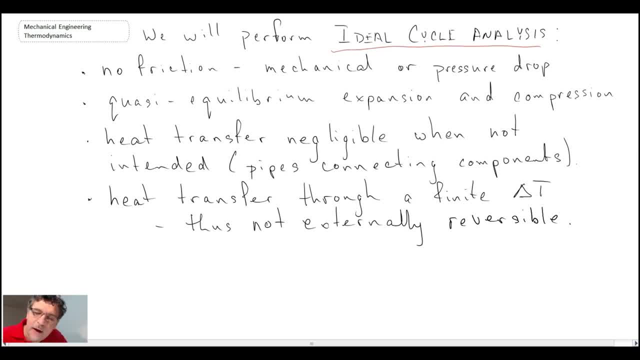 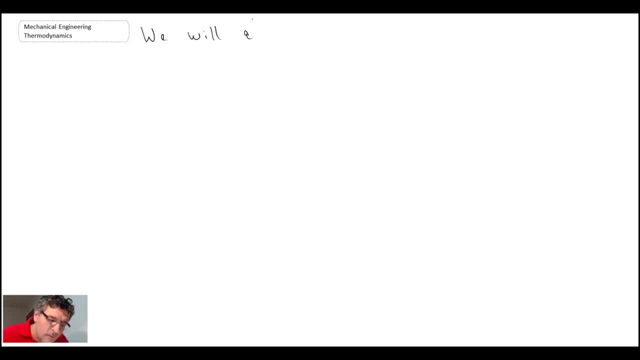 The other set of assumptions that we will make when we look at gas power cycles are called the aerodynamic. These are called the error standard assumptions, And what these state are the following: The first is that the working fluid in our engine is assumed to be air. 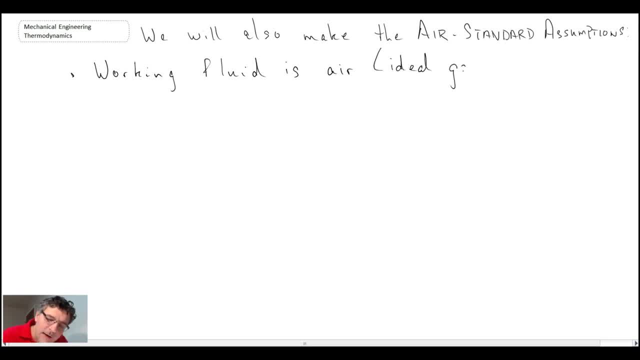 And we'll assume it to be an ideal gas under the conditions that we're looking at And that it circulates in a closed loop. Now we know this is not true, because for any engine the air comes in, fuel is added, it combusts and then it exhausts out. 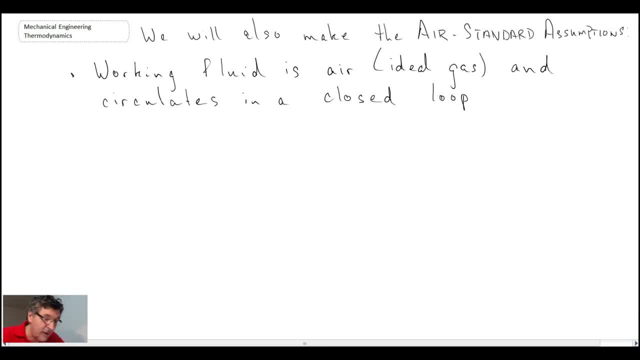 But we're going to assume that it operates in a closed loop. So that's part of the error standard assumption And it enables us to be able to do our analysis. otherwise it would be too complex. Another assumption that we will make is that all cycle processes. 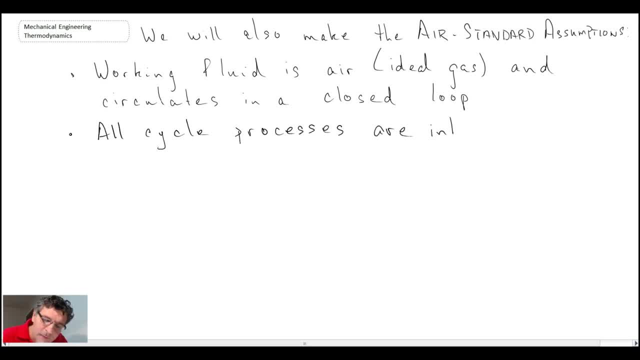 are internally reversible. Now we do have combustion, but we're assuming the working fluid is air and consequently we do not take into account, with this error standard assumption that we have a fuel-air mixture. But what we'll assume is that combustion processes are replaced by 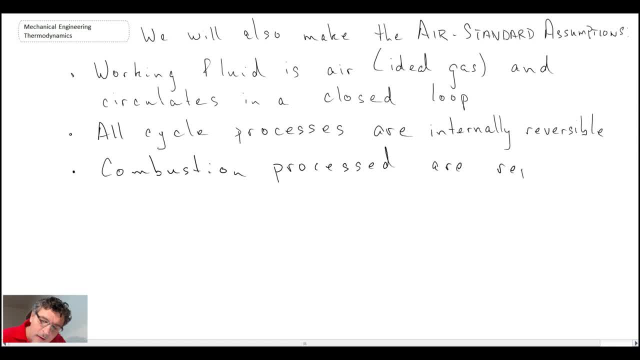 we're going to assume that they're replaced by a heat addition process And we're going to assume that this is coming from an external source. And the other thing that we will assume is that the exhaust cycle or the exhaust component of our cycle. 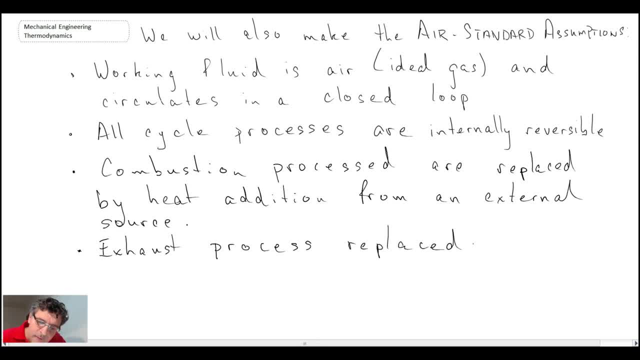 is replaced by heat rejection, And that enables the working fluid then to cool down. In reality, with these engines, what we do is we purge them, And that enables the working fluid then to cool down. We dump it into the atmosphere and we draw in a new, fresh charge of air. 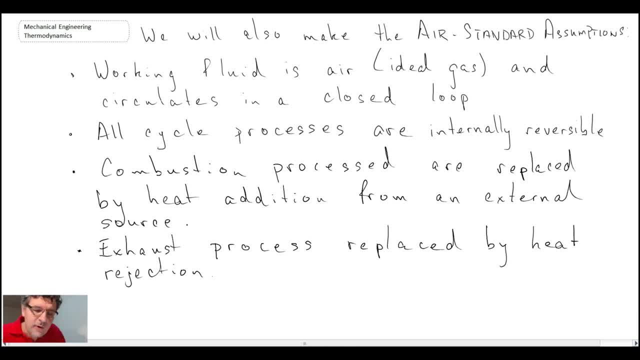 and then we mix it with fuel. But what we'll assume is that there's a heat transfer process that takes place And that enables us then to do a cycle analysis for whatever cycle we're looking at, be it the internal combustion engine with spark ignition.